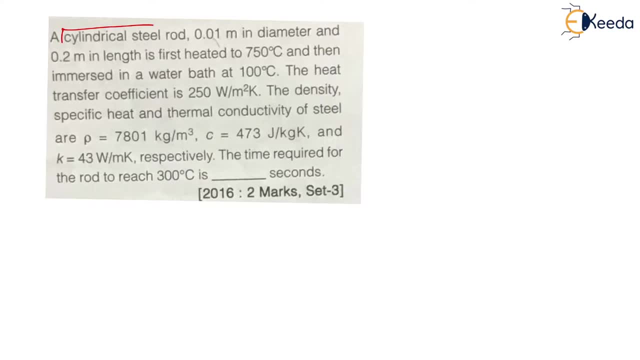 Now cylindrical rod is given. Now, my dear students, they have provided a cylindrical steel rod. So let us draw the diagram Here. cylindrical means it will be having diameter and length red. This is how the rod will look. like red, It will be having some diameter d and it will be having some length l. 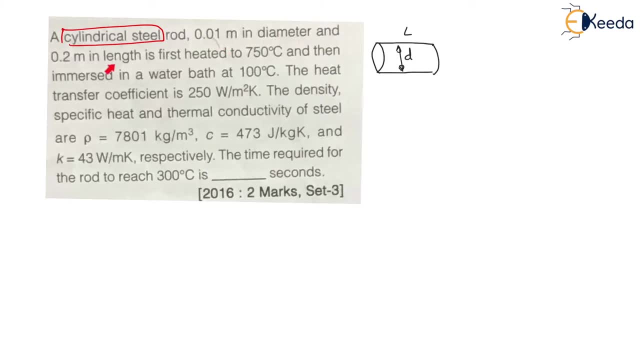 Now here they have mentioned 0.01 meter diameter and 0.2 meter in length. So diameter is given 0.01 and meter and length is given 0.01.. 0.2 meter Then is first heated to 750 degree Celsius. 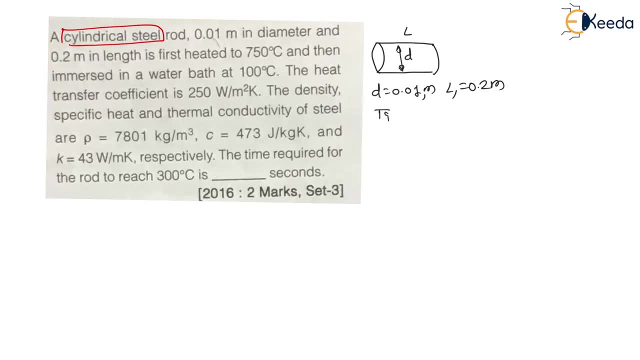 Means it is heated to means its initial temperature of this rod is 750 degree Celsius. Then and then immersed in a water bath at 100 degree Celsius. Now, water bath is nothing but surrounding fluid. The surrounding fluid is at temperature: 100 degree Celsius. 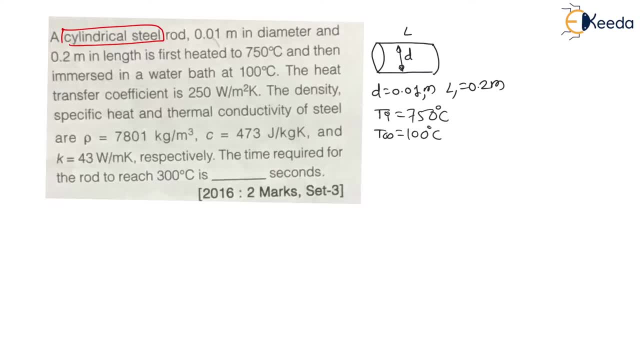 Therefore T infinity is equal to 100 degree Celsius, Then the heat transfer coefficient is 250 V Vat per meter square Kelvin. Here with water, the convective heat transfer coefficient is given 250.. It is 250 Vat per meter square Kelvin. 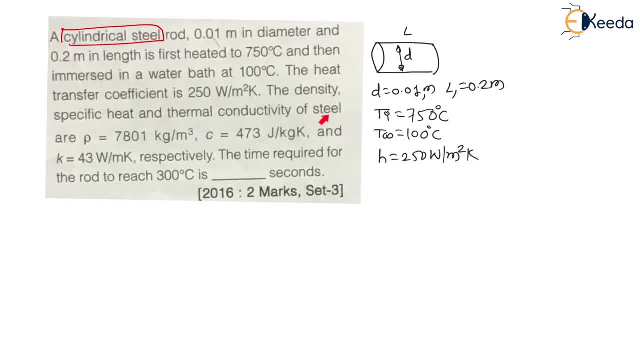 Then the density, specific heat and thermal conductivity of steel are Now here. density is given, It is 7801 kg per meter cube. Then specific heat, C, is given, C is nothing but 473 Joule per kg Kelvin. And thermal conductivity K is given, 43 Vat per meter Kelvin. 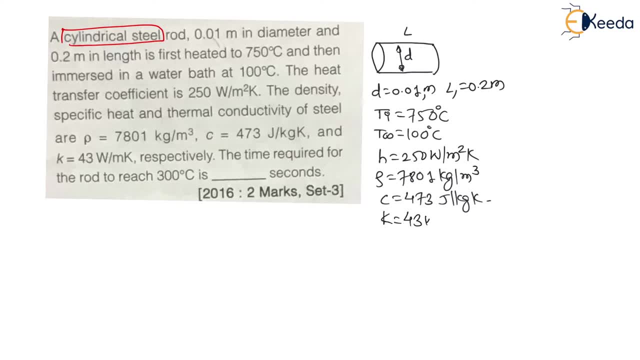 Right. Therefore, thermal conductivity is equal to 43 Vat per meter Kelvin respectively. Now the question is the time required for the rod to reach 300 degree Celsius. is Now, my dear students, what is the time required for the rod to reach 300 degree Celsius? 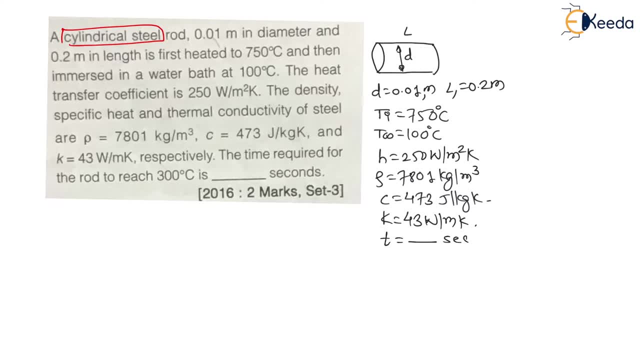 Means time T, we have to find in second, to reach temperature of 300 degree Celsius. For such type of question we have to find first biot number. Now, biot number is nothing but H, L divided by K of solid, Where this L is nothing but characteristic dimension, which is volume divided by surface area. 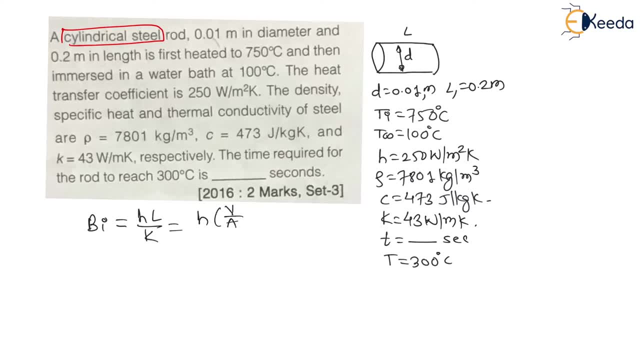 Therefore it will become H into volume divided by area of this cylinder divided by K. Therefore, let us put the values: H into volume is pi by 4, D square into L And surface area is pi D, L for the cylinder divided by K, Here pi D. pi D will get cancelled. 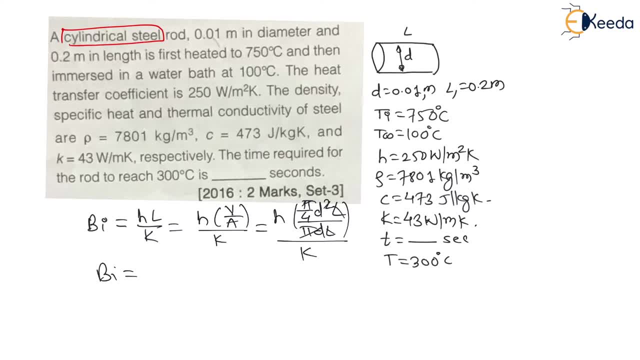 Right, L, L will get cancelled. Therefore this biot number becomes H into D, divided by 4 K. So let us put the values Here. H is given 250.. Diameter is 0.01.. Divided by 4 into thermal conductivity is given 43.. 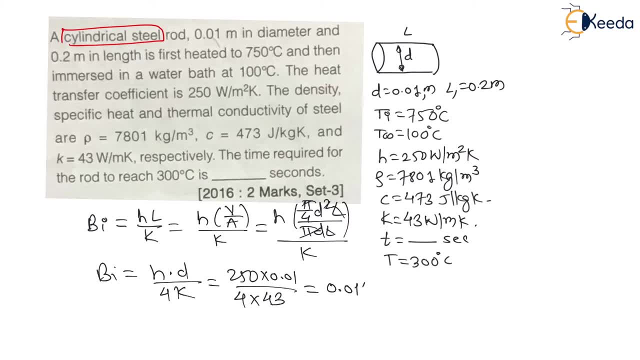 If I find this biot number, I will get answer as 0.0145.. And this answer is less than 0.1.. So, my dear students, whenever biot number is less than 0.1. Then lumped analysis is valid. 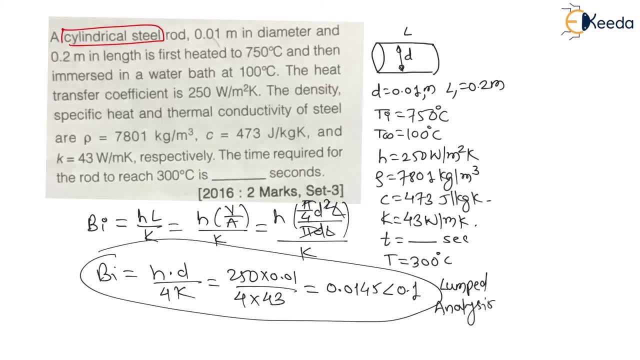 It is a problem of lumped analysis. My dear students, let us use the formulas of lumped analysis to solve this question Right Now. here I am going to use temperature distribution formula for lumped capacity analysis. Now, the formula for lumped analysis is temperature T minus T infinity divided by T i minus T infinity. 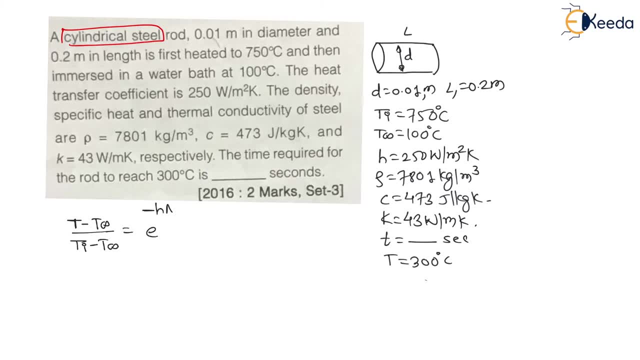 Is equal to e, to the power minus H a divided by rho, v, C, p into T, Where T is the temperature after time, T. T infinity is the fluid temperature. T i is the initial temperature of this object. Here H is convective heat transfer coefficient. 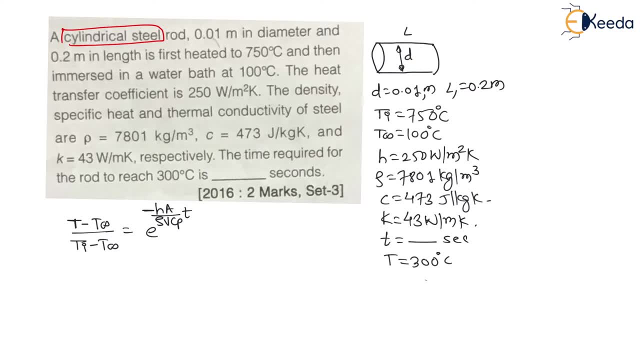 A is the surface area of this object, which is pi, D, L, V is the volume of this cylinder, Rho is density of this cylinder, C, p is specific heat of the cylinder And T is the here time. So let us calculate first area divided by volume. 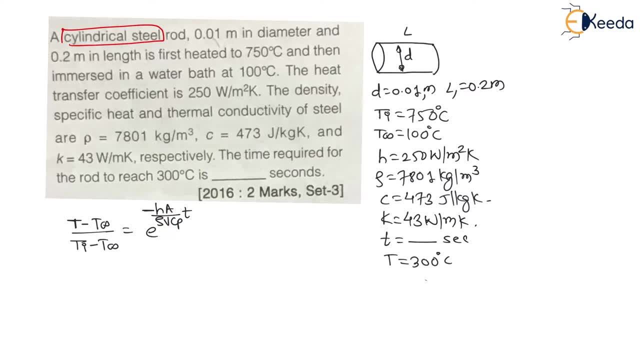 Just now. we have calculated few minutes back, while deriving the biot number formula. In biot number formula, we have calculated volume. We have calculated volume divided by area. Now here let us calculate this area divided by volume. Area of the cylinder is pi D, L. 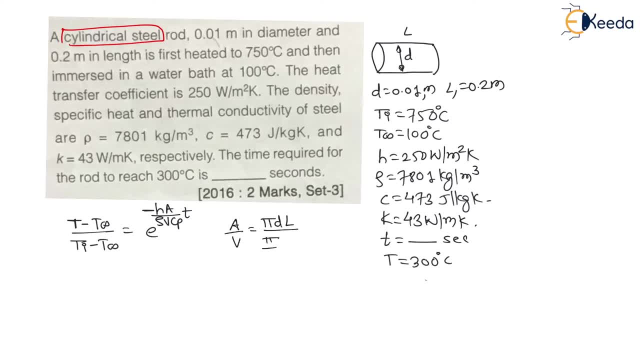 That is surface area for the convection, And volume is pi by 4 D square L. So here pi, pi, D and L will get cancelled, So it will remain 4 by D. Right, That is area divided by volume. I can replace with 4 divided by D. 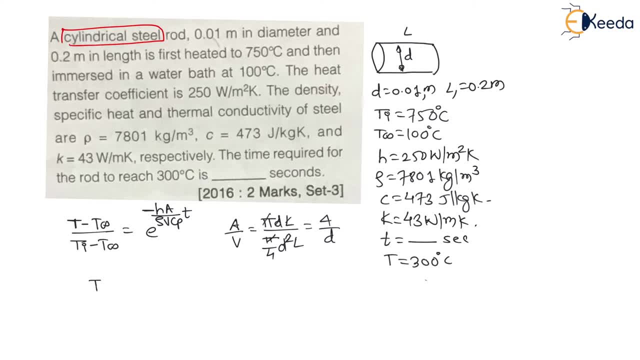 Therefore replace here in the formula. Therefore we will get formula T minus T infinity divided by T i minus T infinity, Right? So here pi D is equal to minus H p divided by rho C p, And this area divided by volume will become 4 divided by diameter. 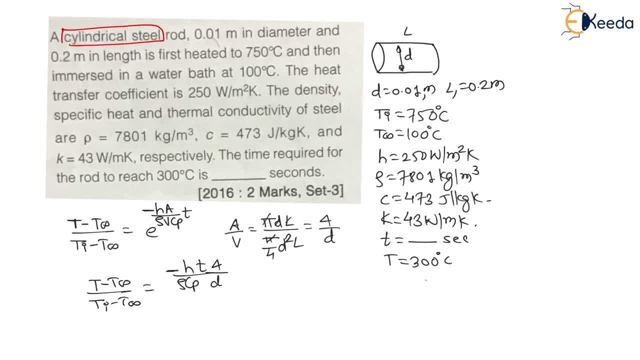 Right Now, let us put the values in this formula. Therefore, my dear students, temperature is given 300 degree Celsius. Therefore, 300 minus T. infinity Surrounding fluid temperature is 100 degree Celsius, Right Minus 100.. You have, a initial temperature is 750. 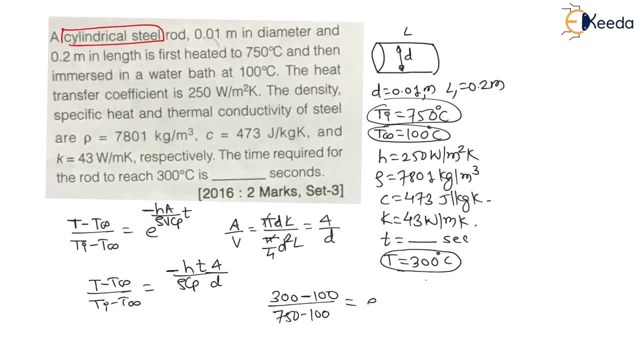 750 minus 100 is equal to e, to the power Minus H, H is 250.. Minus 250. Into time is we have to calculate into 4. Divided by Density is given 7801. into specific heat, is given 473.. 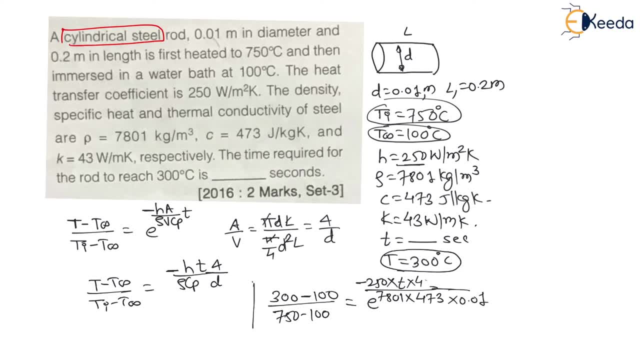 Into diameter is 0.01.. Right Now, my dear students, in this complete equation only time T is unknown. So let us solve this equation. for finding T Right Now, if I consider Ln on both sides, Then this exponential function will go. 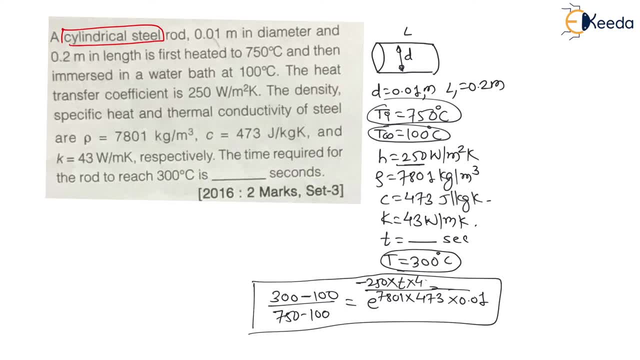 Vanish Right. Therefore, let us write here answer. Therefore I will get answer. as 200 divided by 650 is equal to e, to the power minus 0.0271 into time T Right. Let us consider Ln function on both sides. 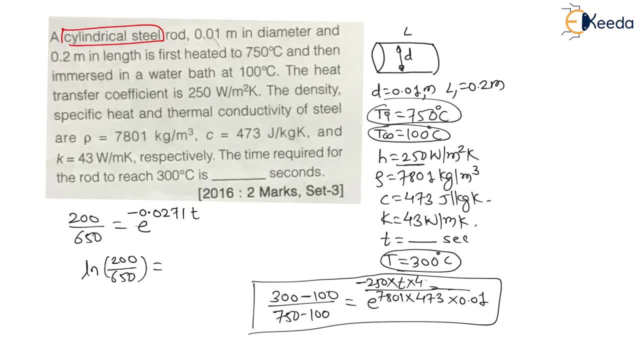 Therefore, Ln of 2000 divided by 650 is equal to minus 0.0271 T. Right Now, let us solve this equation for T. If I calculate T, I will get time as 43.65 second. This will be time. 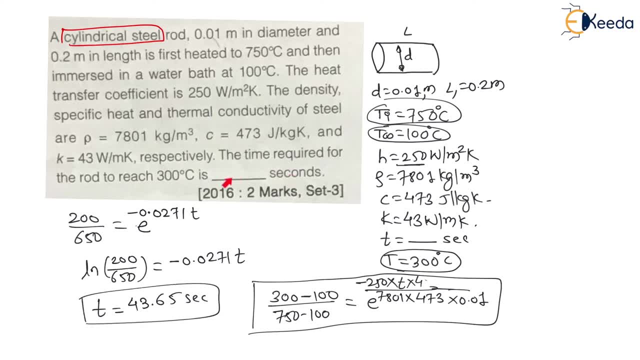 Right. So my dear students, here they are asking time in second. Therefore, in this bracket you have to type 43.65 for getting full mark. Therefore, your answer is 43.65.. Thank you, dear students. In next lecture we will see one more numerical on this topic which was asked in previous year.